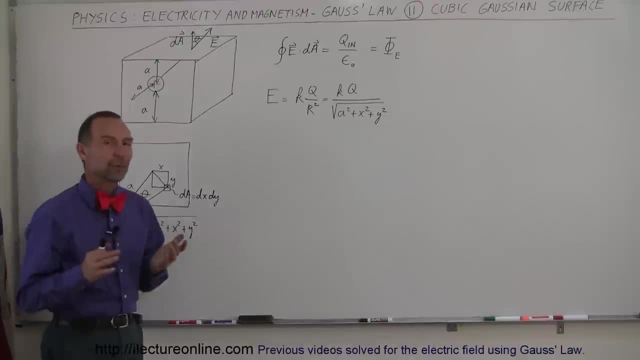 Welcome to Electron Online, and now we're going to take a look at Gauss's Law in a different way. A lot of my students always ask: why do we have to put spherical or cylindrical Gaussian surface around our charges? Why can't we just put a cube around our charges? And here this video is. 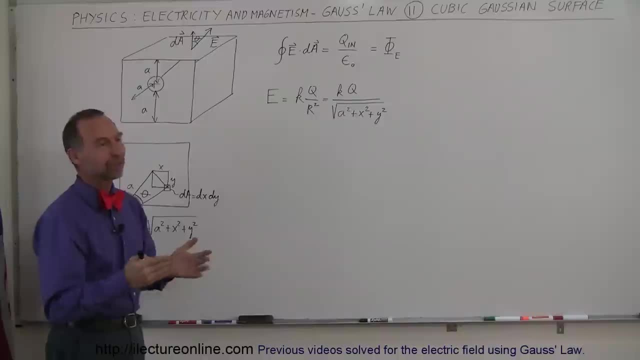 made to let you know why you shouldn't try to put cubic Gaussian surface around charges to find the electric field strength at a particular distance. So let's say we have a point chart right here that has charge q on it. Let me just write it. and let's say that we put a cubic Gaussian surface around. 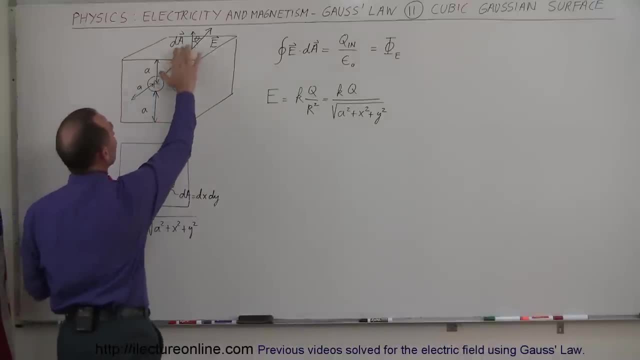 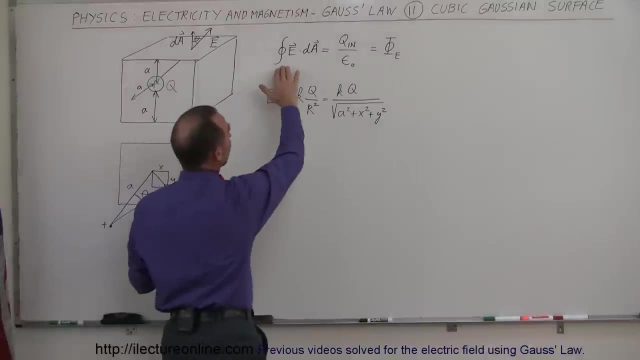 that charge and we want to find what the electric field strength is at any point in along the surface of that Gaussian surface. Well, what you want to do is, of course, use the Gaussian equation, the Gauss's Law equation. We have the surface integral of e. dot dA equals the q inside divided. 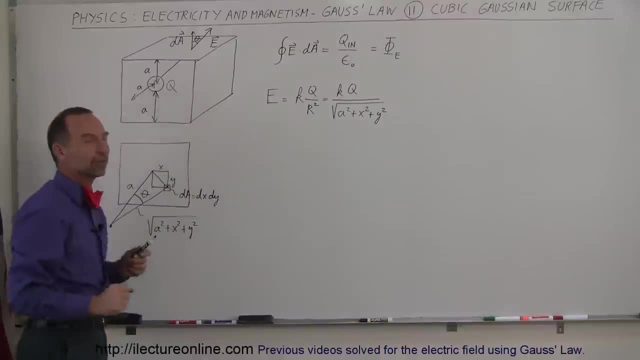 by epsilon sub zero, q. inside is simply q. epsilon sub zero is our constant. but now what about the e dot dA? Now notice that the direction of the dA will always be perpendicular away from the surface and, of course, as you get to certain points on the surface, the electric field will be away. 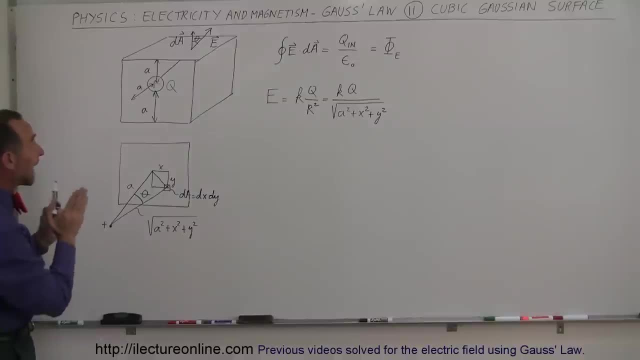 radially away from the central charge, and you can see now that there's going to be an angle between them. let's call the angle theta. So what I did was I took this surface right here, I folded it up like this: here's our charge at the center. now we're looking from the center of the cube. 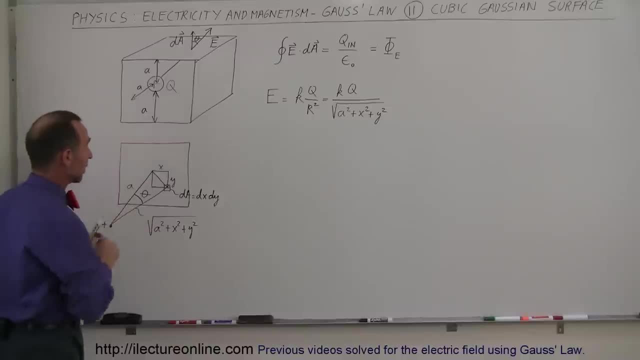 towards one of the faces and of course it wouldn't matter which face you look at, you get the same kind of idea. This is the central point of the face, directly above the charge. So you can see that this line from there would be perpendicular to the surface. 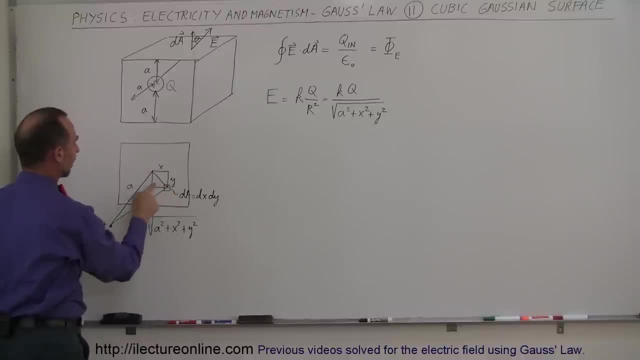 Let's pick a point away from the center, this point right there, and so let's draw, let's try to find the distance from the charge to that point on the surface. Now notice that the distance from there to there- I called it a A- would be half the distance from the well would be the distance. 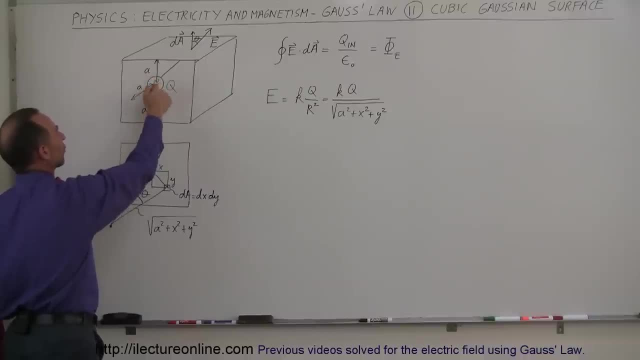 from the central charge to the side in any direction. So from there to the front face, from there to the bottom face, from there to the top face, is a. So that's this distance right here. trying to find this distance over here, Notice that we have a distance x away from the center in. 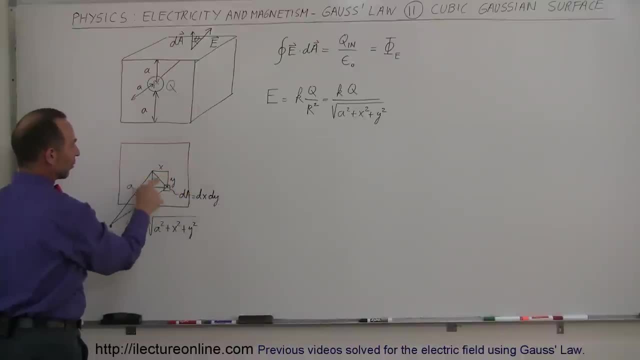 this direction and a distance y away from the center in this direction. So this here, this line across here, would be x squared plus y squared. There we go and then you notice also that this diagonal distance here is the square root of a squared plus x squared plus y squared. 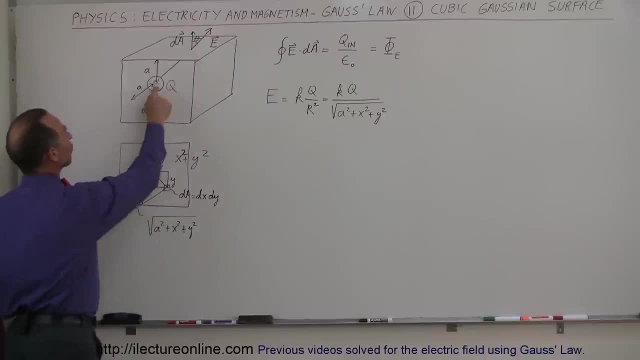 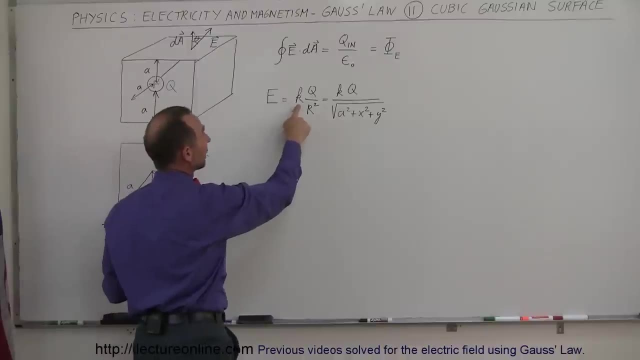 So that would be the diagonal distance right here. that would be the distance from the charge to any random spot on the surface. Now the electric field strength at that point would be equal to k times q divided by r squared, and r squared, of course, is kq over. 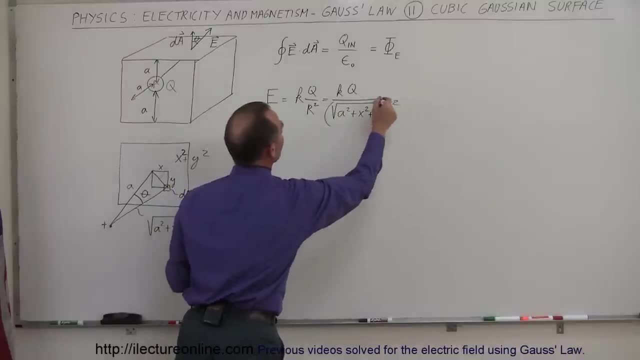 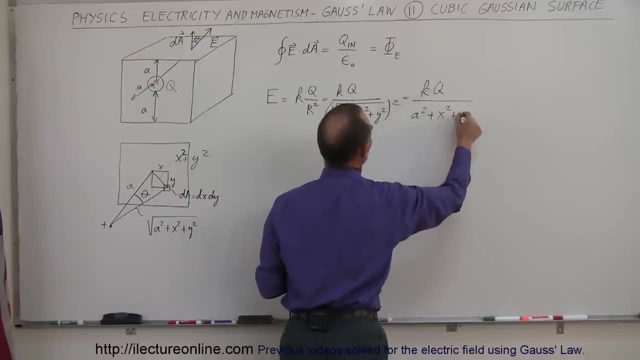 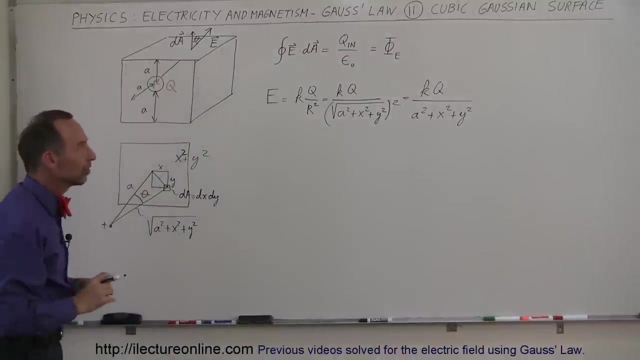 this distance, and of course we have to then square that like that, So you can write this as: k times q divided by a squared plus x squared plus y squared, That would be the strength of the electric field anywhere along, anywhere on the surface or one of the faces of that cube. 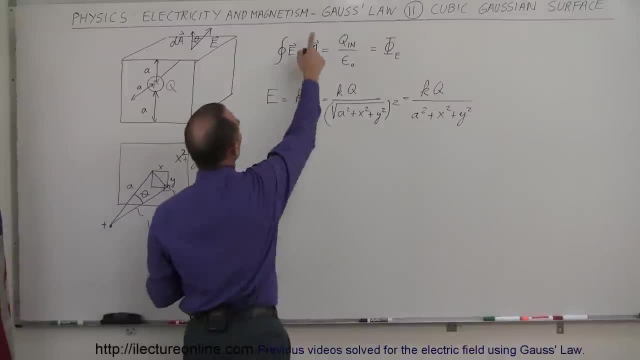 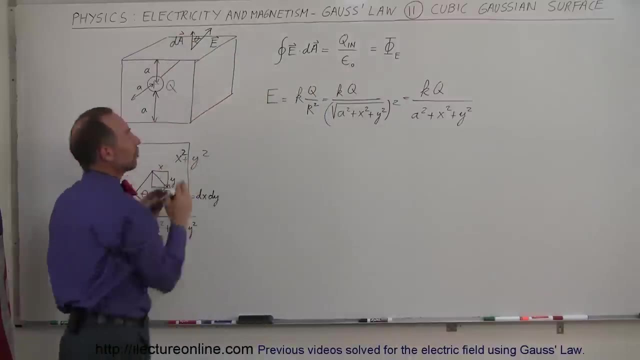 So now also realize that the that the integral e, dot d, a would, would give you the flux, electric flux going to the side, and since there's six cubes and each cube is the same distance away from the central charge, each phase would have one-sixth of. 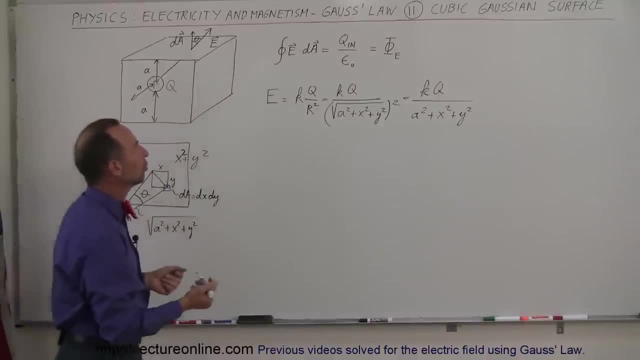 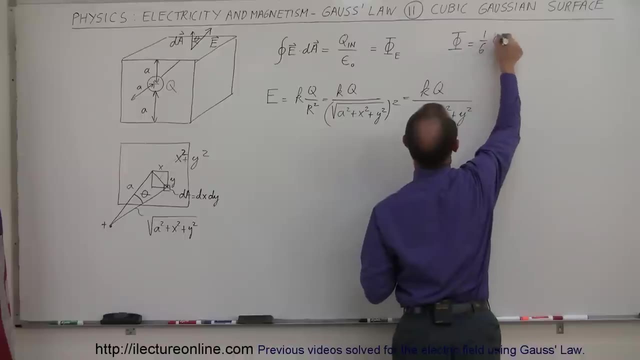 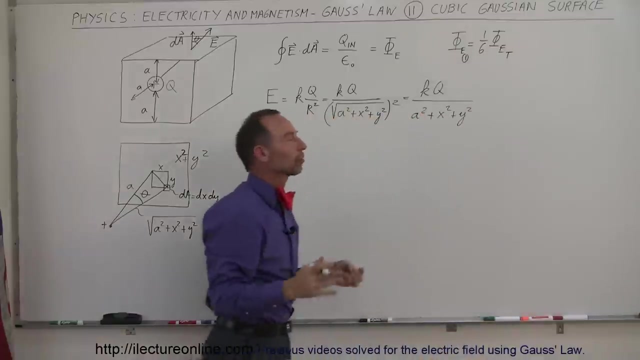 the total electric flux to that. So we can assume that the electric flux through one of the phases is equal to one-sixth the electric flux, total, electric total. So that would be electric through one of the phases would be one-sixth the total flux. 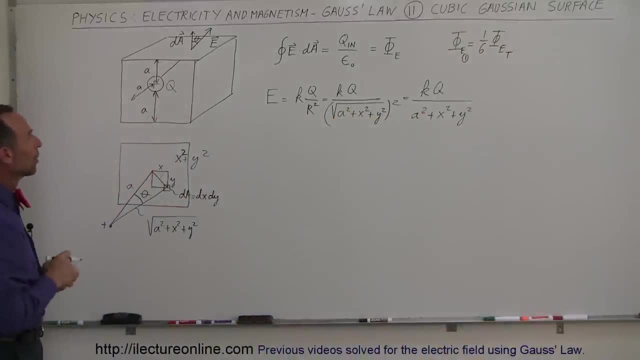 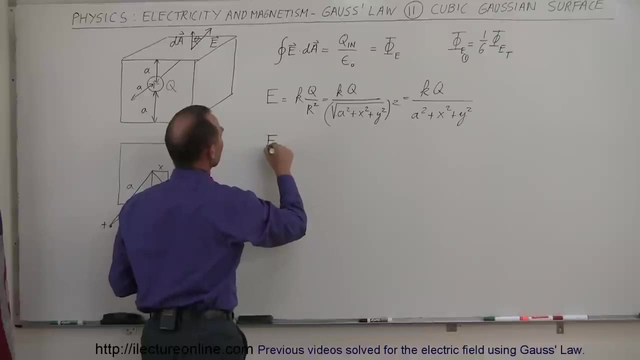 Going through all the sides. all right now. what we want to do is we want to go ahead and calculate what e dot d a is. Well, we know that e dot d a, or e times d a, is equal to e times d a times the and. 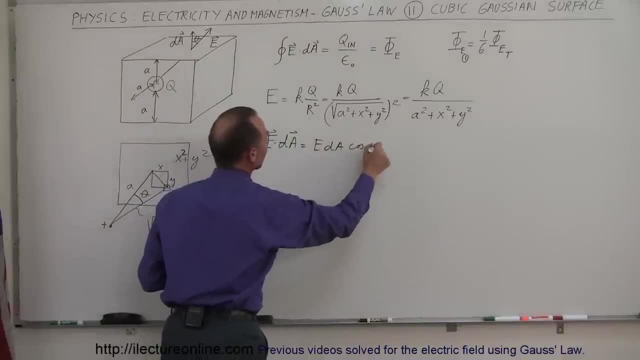 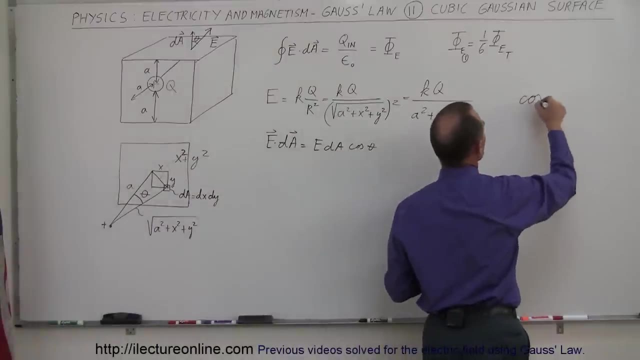 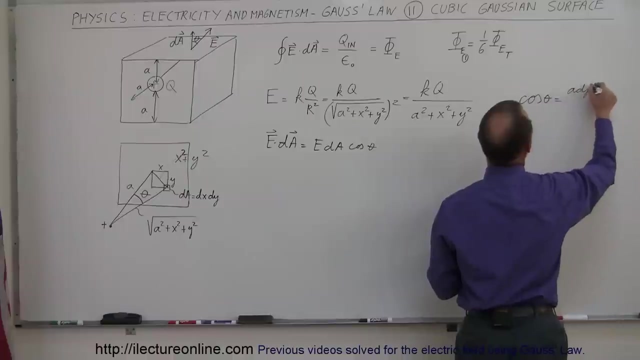 of course I do it like this times- the cosine of the angle between them. Now, how do we find the cosine of the angle between them? Well, let's see here. the definition of the cosine is equal to the adjacent side divided by hypotenuse. That would be the ratio of the adjacent side divided by the. 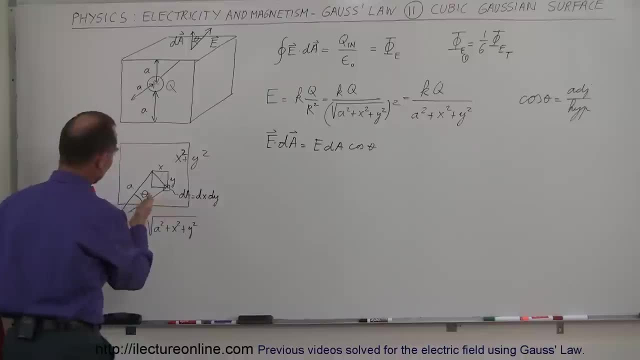 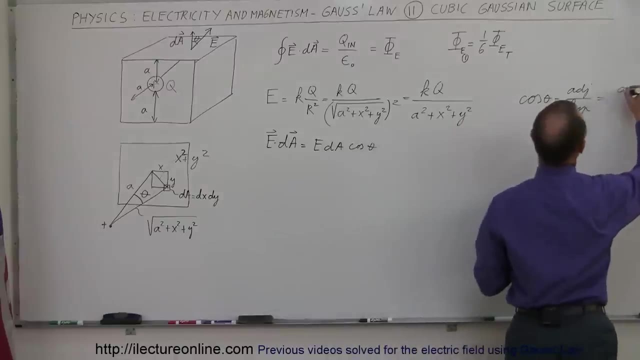 hypotenuse, And here you can see that the adjacent side would be a and the hypotenuse, of course, would be this quantity right here. So we can write this as a divided by the square root of a square plus x square plus y square. That would be the cosine of theta. So we can write e dot, d a times the. 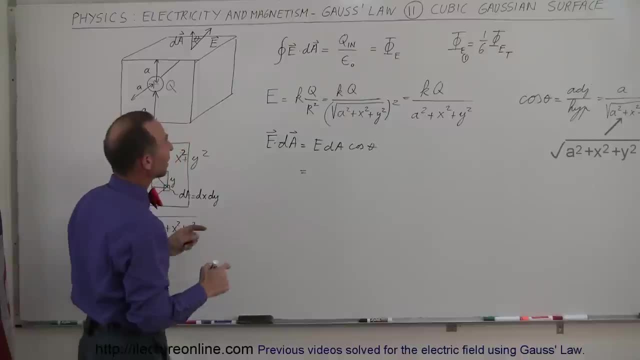 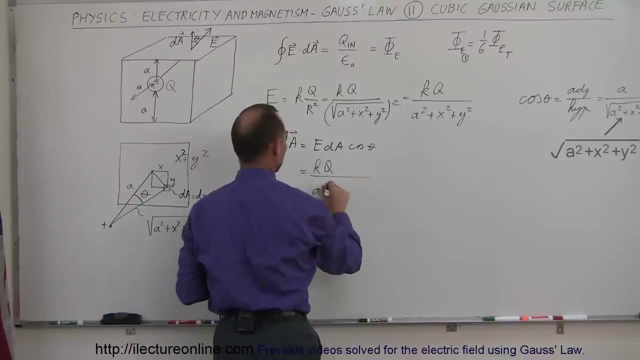 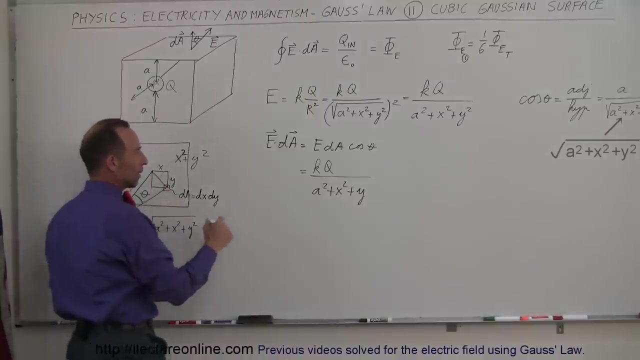 cosine of theta equal to e, of course, would be equal to this quantity right here. So it would be k times q, divided by a square plus x square plus y square d a- that's a small little area element- right here simply would be d x times d y, So it would be d x times d y and the cosine of theta would be equal to. 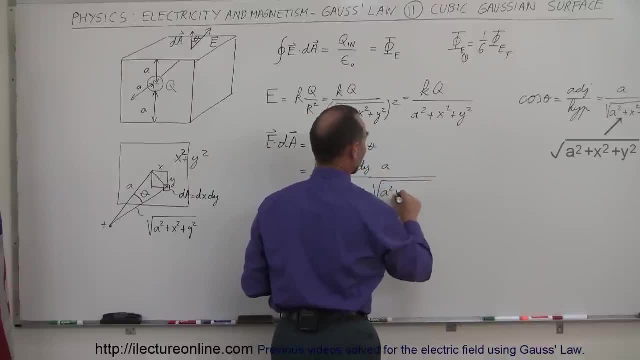 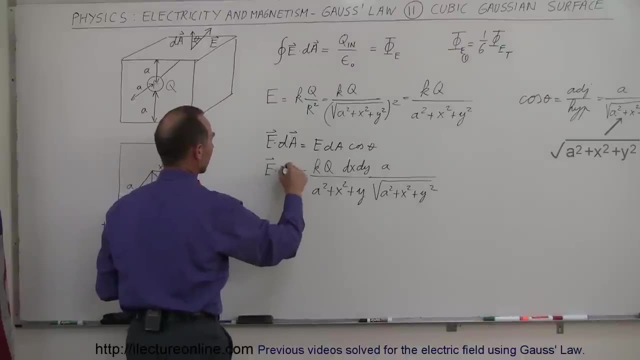 a divided by the square root of a square plus x square plus y square- Okay, that would be e dot d. a times q divided by a square plus x square plus y square, Okay, that would be E dot dA. And if we now want to integrate that, so the integral of E dot dA would be equal to the integral of this. 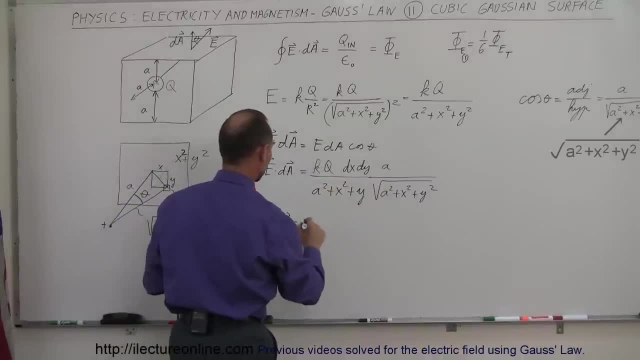 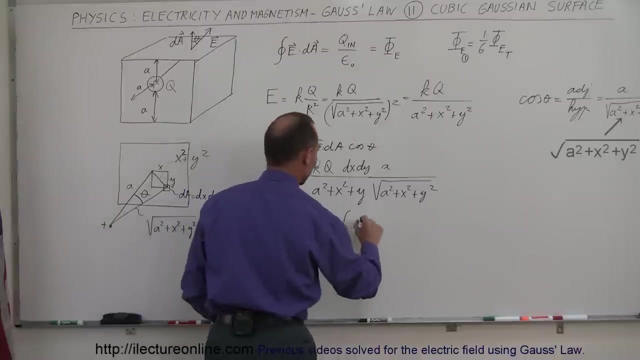 Now notice that A is a constant, K and Q are constants, so this could be written as the double integral or the surface integral, I should say the surface integral of. well, let's see, let's get the constant out first. it would be KQ times A times the surface integral of dx times dy. 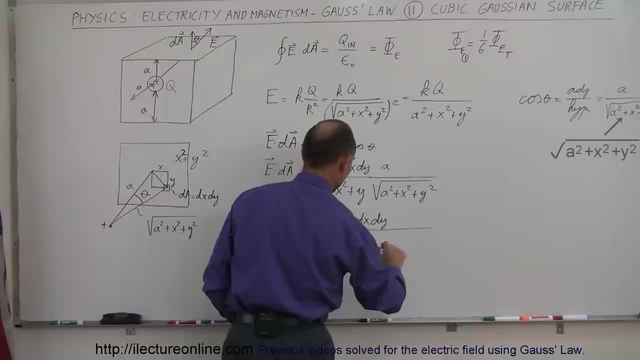 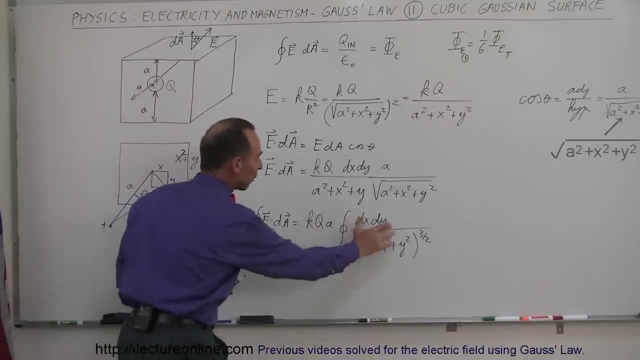 divided by the quantity A squared plus X squared plus Y, squared to the three-halves power. And now this would then become a double integral over the X and the Y to integrate over the entire surface, And of course we know that this is equal to the flux through. 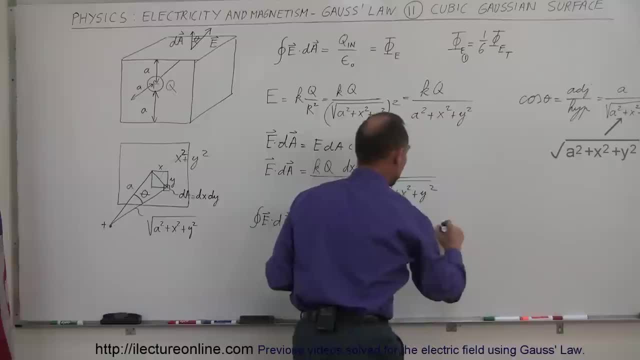 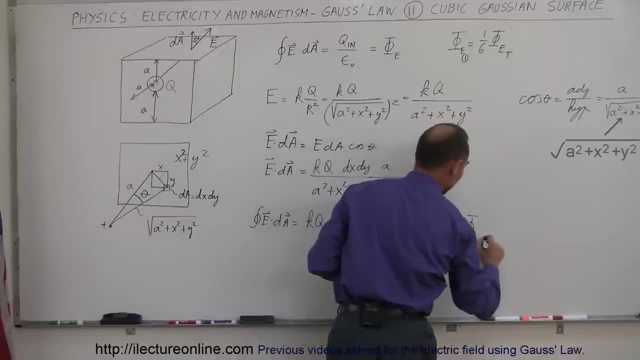 is equal to the flux through the surface. so that would be equal to one-sixth the total electric flux emanating from this charge. so that would be total electric flux. And then, of course, from Gauss's law we know that the integral, which is equal to the electric flux, 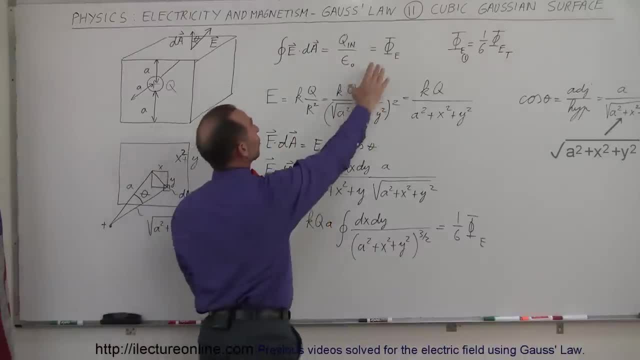 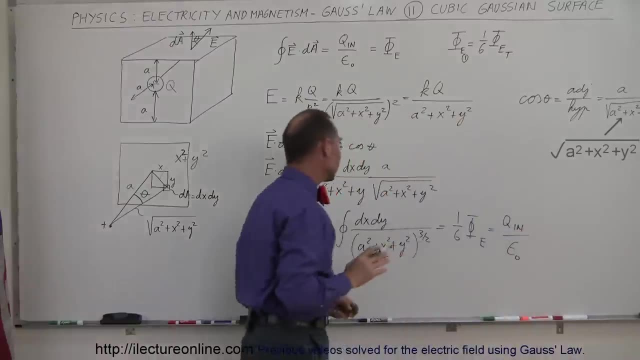 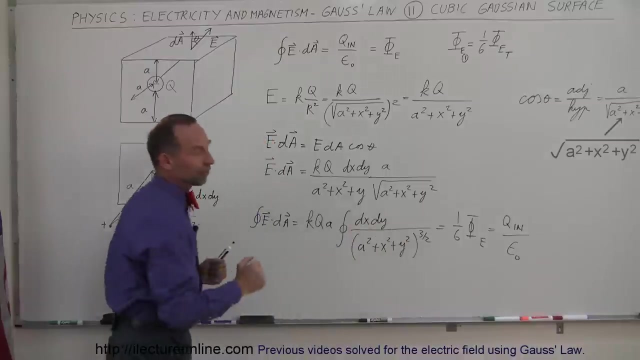 in this case the one of the surfaces would only be one-sixth of the total flux would be equal to Q inside. Q inside divided by epsilon sub naught. So notice that if you're trying to find the electric field strength using this right here, you're going to be up against a very difficult integral.